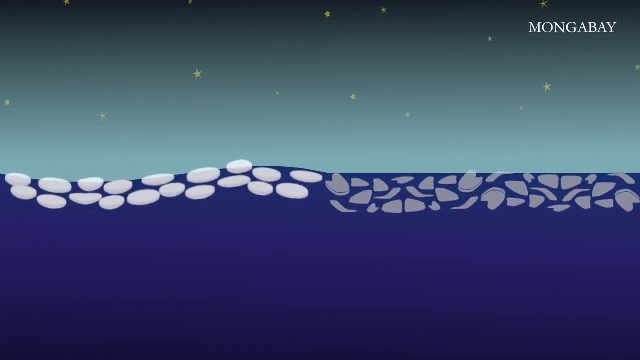 hand, the ice forms rafts that crash into each other, rounding them into thick disks called pancake ice. Eventually, these sheets solidify into flows. These might be smooth and flat, or rough and uneven. Gradually, more ice accumulates on the underside to form first-year ice. 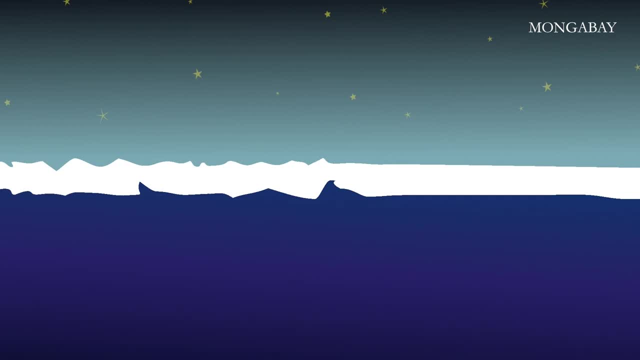 First-year ice can be up to a meter thick. It's salty, brittle, relatively easy to melt and relatively easy to crack. Wind and water currents drive the flows into one another. Where they crash together, they form pressure ridges that rise up to 12 meters high. 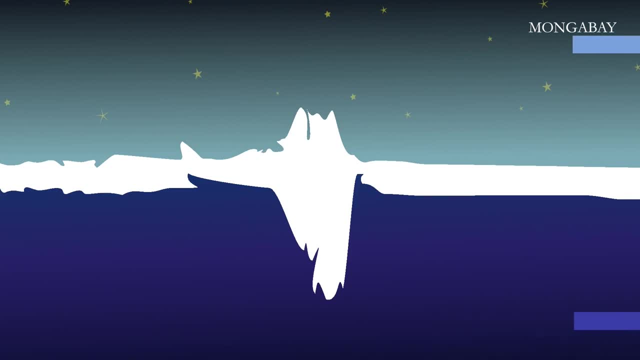 and extend even further below the surface. When ice sheets break apart, they leave narrow cracks called flaw leads. Elsewhere. winds or columns of rising warm water open up larger areas known as polinias. Polinias are like giant lakes in the middle of the ice, expanding and contracting in size, One of the largest in the Arctic. 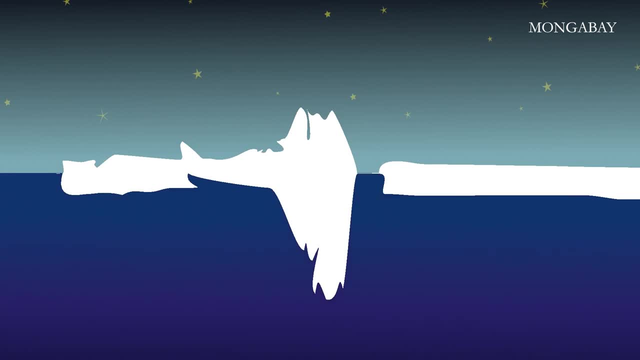 the North Water. Polinia, adjacent to Greenland in northern Canada, can cover up to 85,000 square kilometers, That's about 53,000 square miles. Flaw leads and polinias are crucial to life in the Arctic Algae and other types of phytoplankton flourish here Arctic cod, seals, walrus, polar bears and 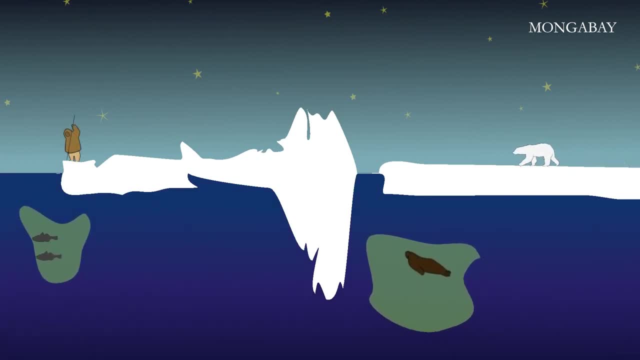 other animals feed. here, Indigenous populations rely on flaw leads and polinias for navigation and hunting. Some of the world's most northern communities live on the edge of the North Water Polinia. As the ice freezes and becomes thicker, it expels salt into the water below That salt. 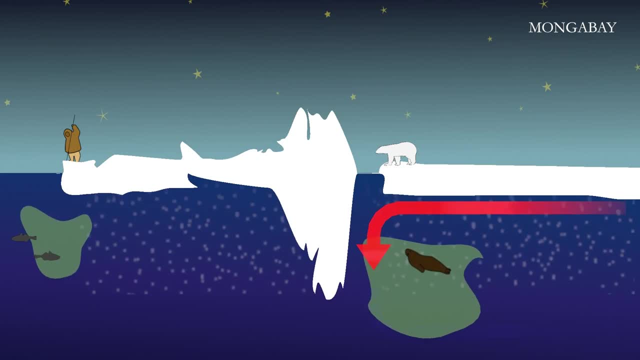 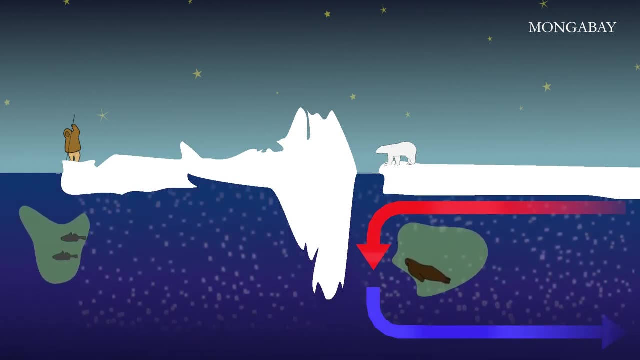 mixes with water from the Atlantic, causing the water to sink and eventually return south. This movement is a crucial part of the global circulation of ocean water that helps regulate Earth's temperature. Salt is expelled upwards, too, in the form of frost flowers. These are 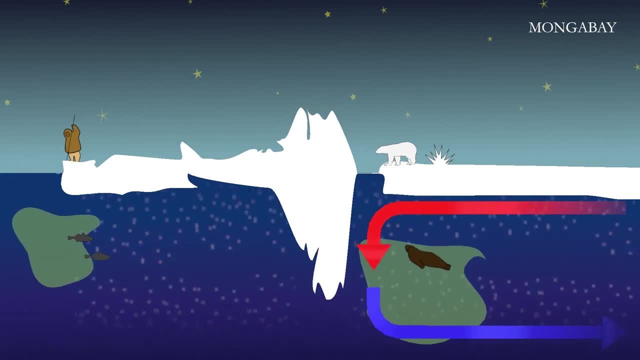 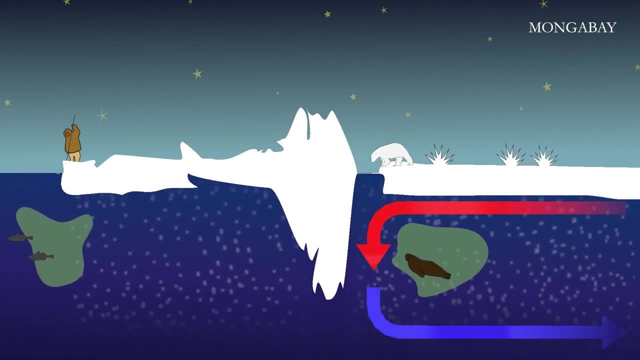 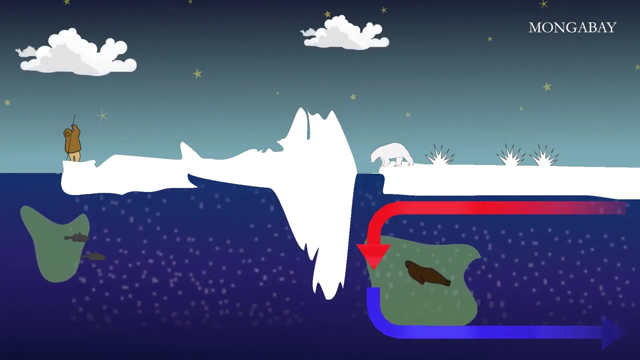 delicate crystalline structures composed of salt and water vapor that freeze in the cold air. Frost flowers used to be rare, but changing conditions in the Arctic have made them more abundant, with some flows of first-year ice covered in the structures. Clouds often form above flaw leads and polinias, It's thought 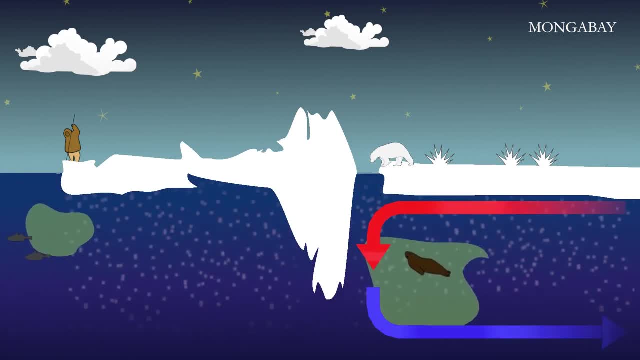 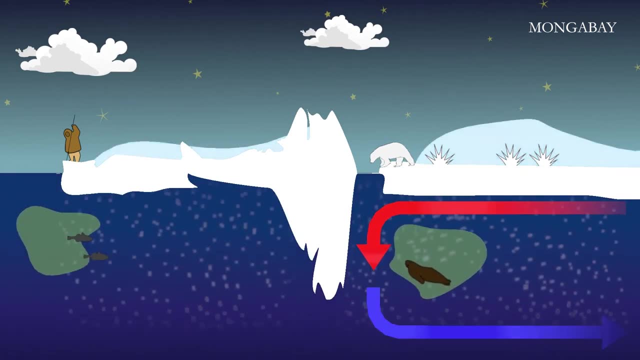 that frost flowers may play a role in the formation of small aerosol particles around which vapor condenses to make clouds. Clouds deposit snow on the ice surface. Frost flowers can trap blowing snow, thickening the snowfield Ice that survives the first year thickens. 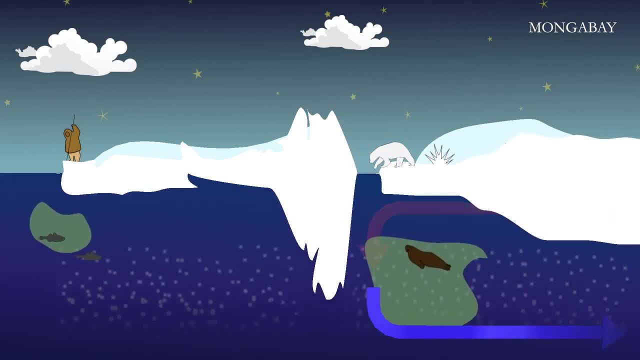 into what's called multi-year ice. Most of the salt has been expelled, making the ice much harder and resistant to breakage and melting. Multi-year ice can be two to four meters thick. It used to be that much of the Arctic Ocean was covered in multi-year ice. 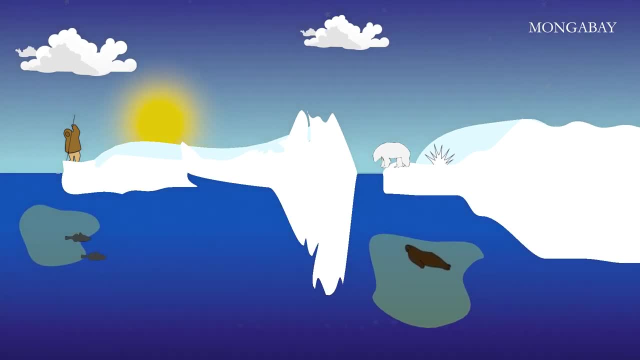 Unfortunately, there is almost none of the thickest multi-year ice remaining in the Arctic Ocean Today. it's almost all fragile first-year ice, which is taking longer and longer every year to form. The main reason for this is that ice is white and reflects the sun's radiation. 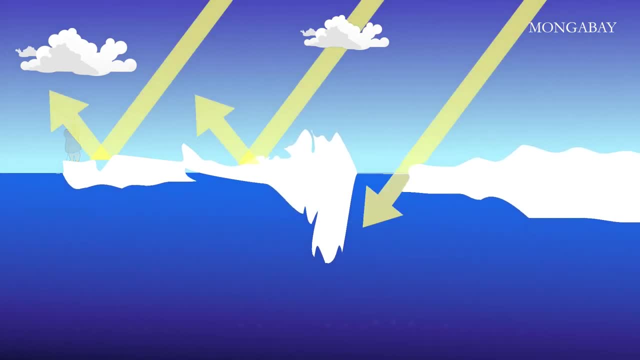 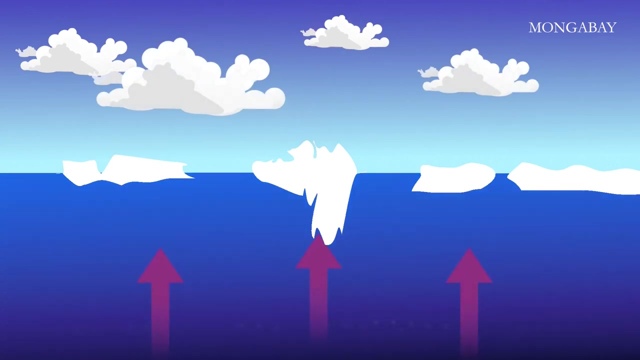 back out into space, keeping the Arctic cool, But darker open water absorbs heat. Global warming is heating the Arctic, Melting the sea ice, creating more dark open water and causing even more ice to melt. There's many other complex factors contributing to the Arctic warming and causing sea ice to 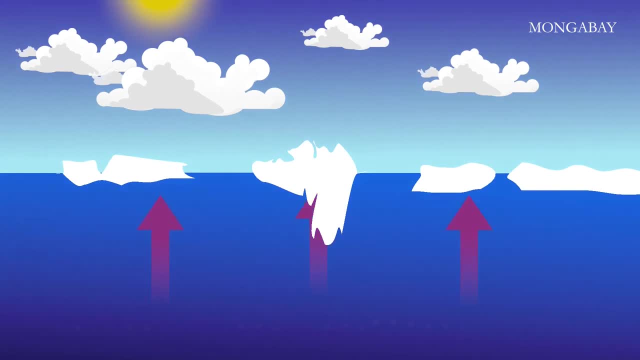 be lost. Wind and wave action, storms and changing water currents are just some examples. Clouds, too, play a role. Although they can reflect sunlight just like ice, in the wintertime clouds act as a blanket trapping warmth. Global warming is most visible in the summertime. 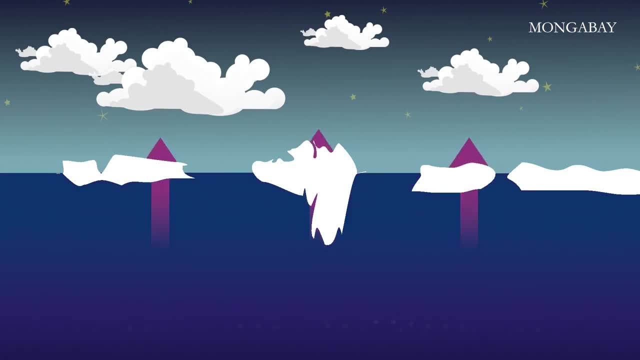 when more and more ice melts, But the Arctic is actually warming fastest in the winter. It is predicted that at the current warming rate, the Arctic could lose all summer sea ice at the latest by 2100, or as early as 2030.. But the complex Arctic climate system 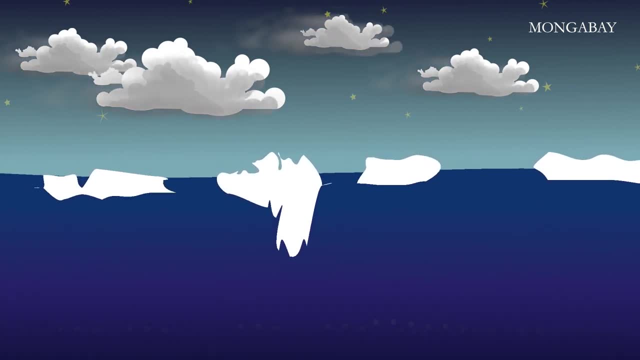 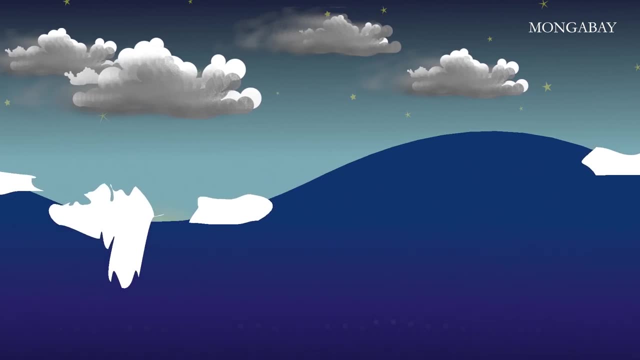